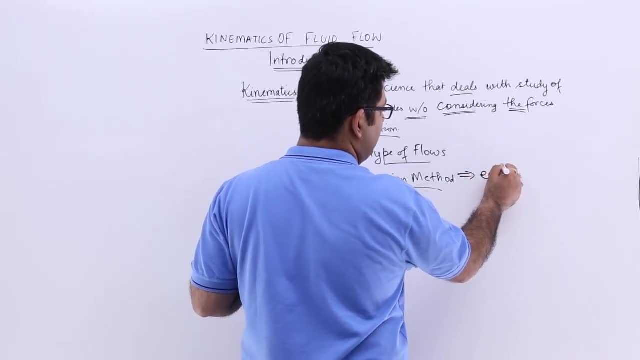 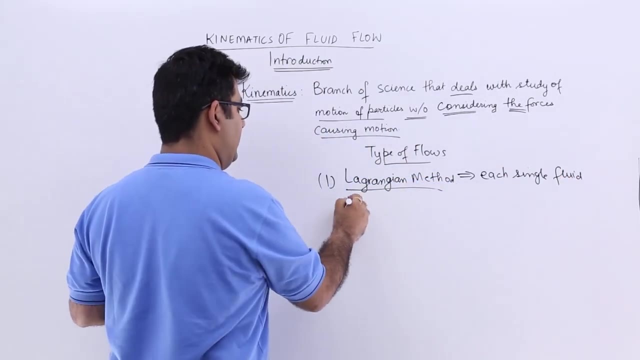 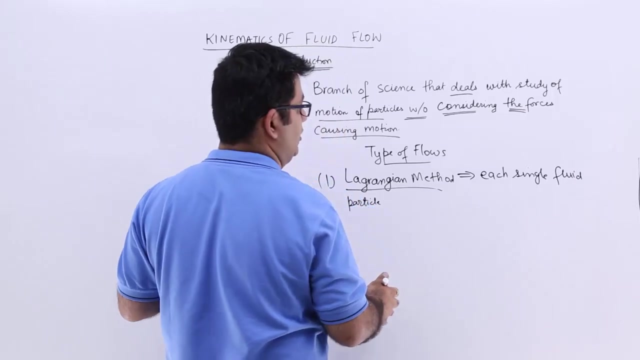 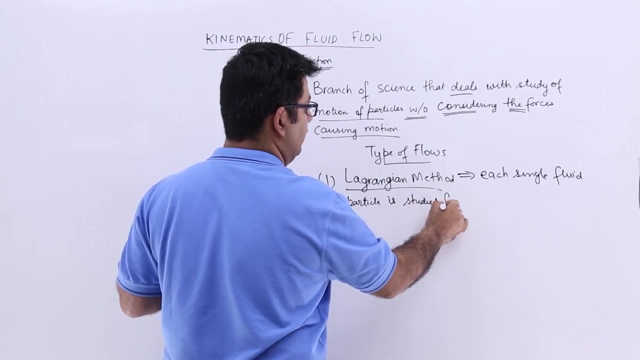 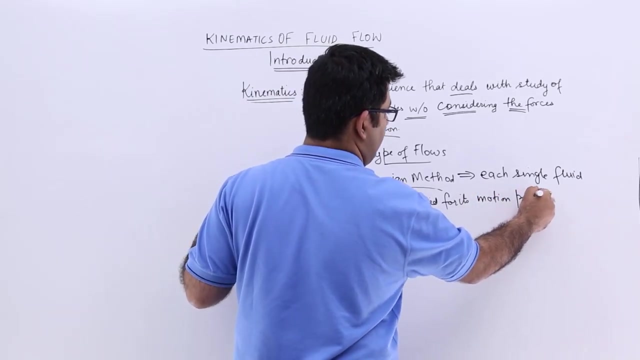 Okay, so in this each single fluid particle is considered, or I would say studied, for its velocity pressure and all the motion characteristics. So single fluid particle is studied for its motion characteristics or motion properties, And these motion properties are nothing but your, as I told you. 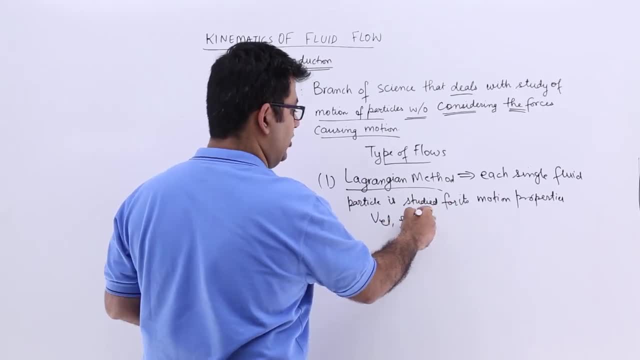 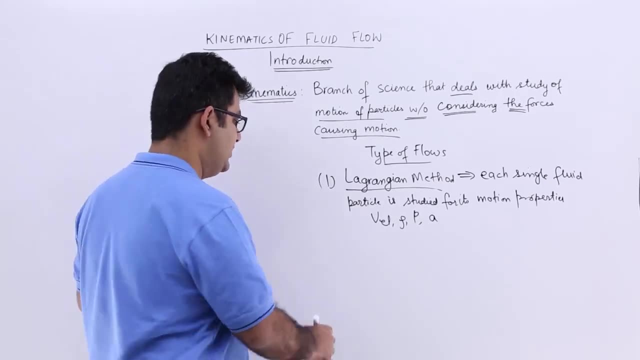 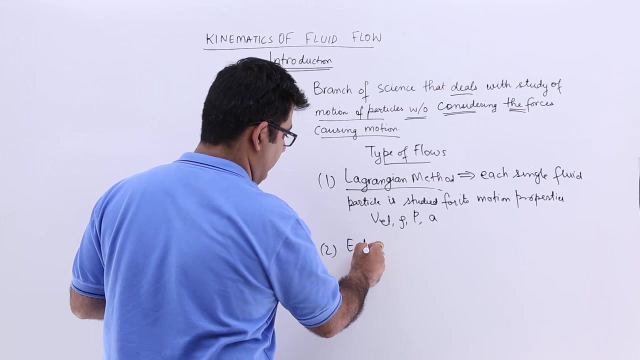 You need to have a velocity, you should have some density, you will have some pressure, some acceleration, etc. Okay, so each and every particle is studied. The second method of describing a fluid motion is the Eulerian method, So it was proposed by Euler. 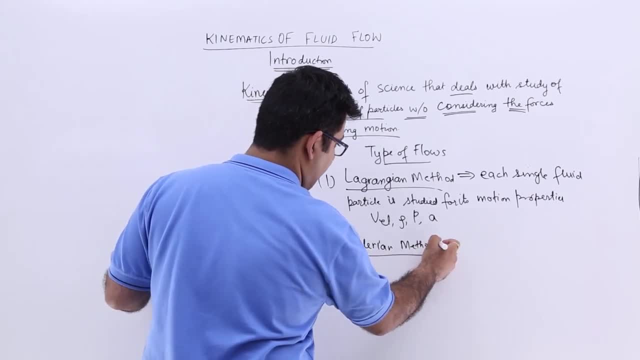 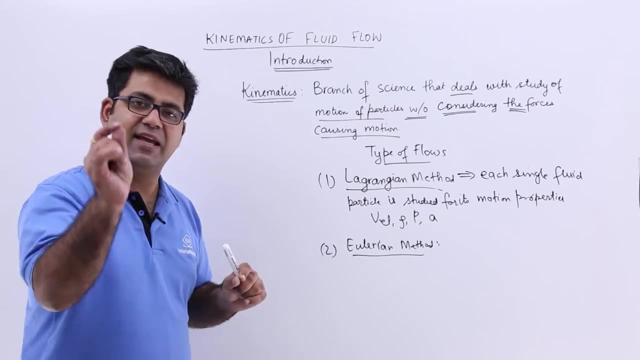 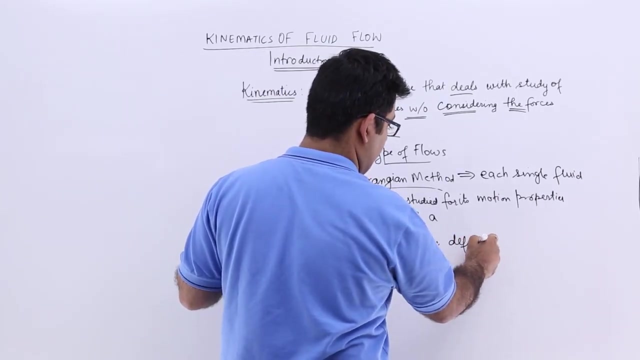 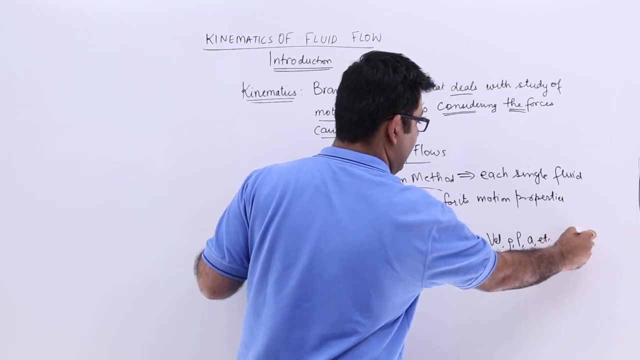 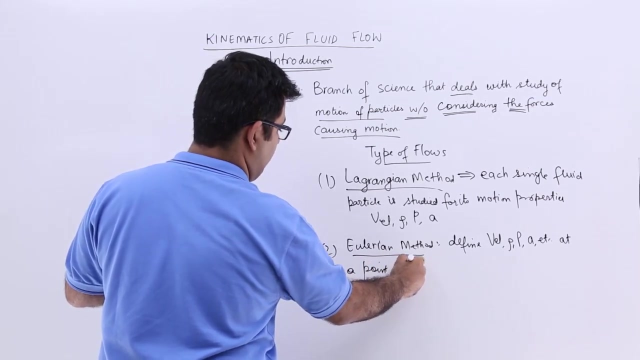 Okay, in this what we do, we define the flow characteristics, the motion characteristics of of a fluid, at a single point in the entire flow field. Okay, so we define. we define velocity, density, pressure, acceleration, etc. at a single point in the entire flow field. 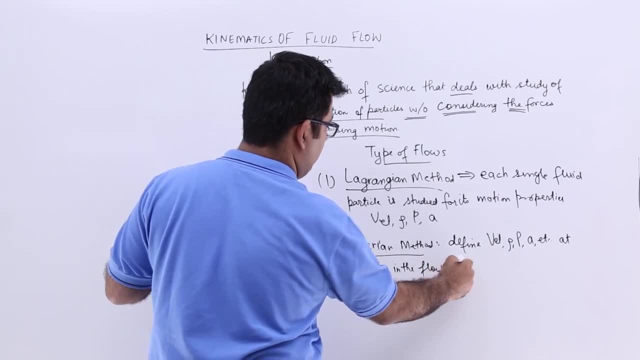 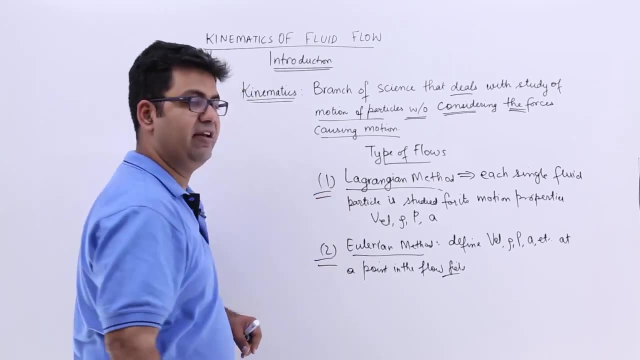 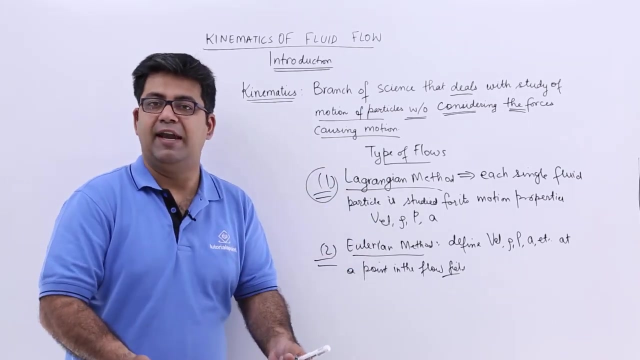 In the entire flow field. So we do not. we do not go after each and every particle in this method, But we go after each and every particle in this method. Okay now, but obvious. this is very difficult to, you know, carry out, But to make use of the Eulerian method, it's very easy. 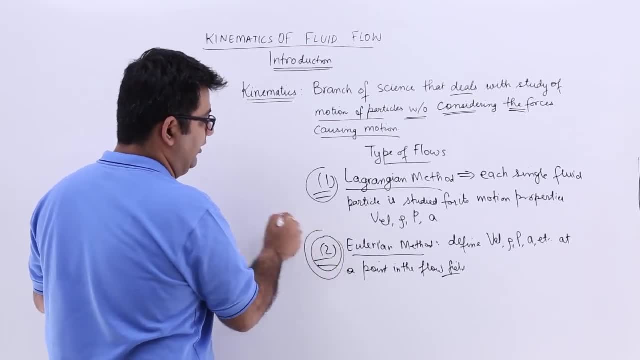 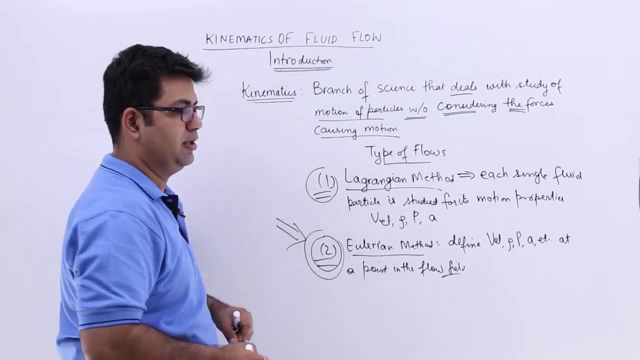 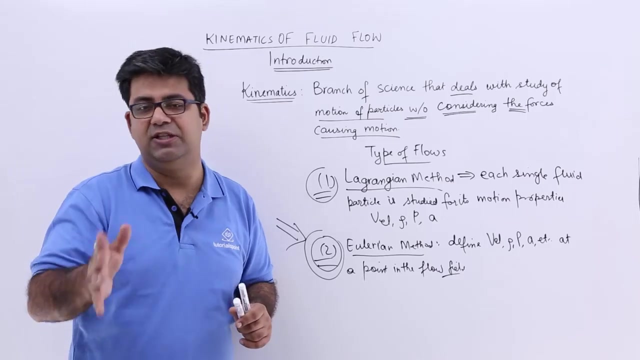 So in most of our analysis that we are going to study in this chapter of kinematics of fluid flow, We will consider the Eulerian method of describing a fluid flow. Okay, so I hope you got a basic idea what we are going to deal with in this particular chapter. 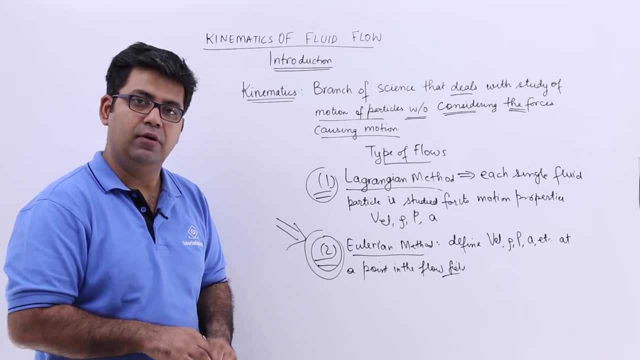 So now let's move on to the next video and talk about the different type of flows that we encounter in daily life.